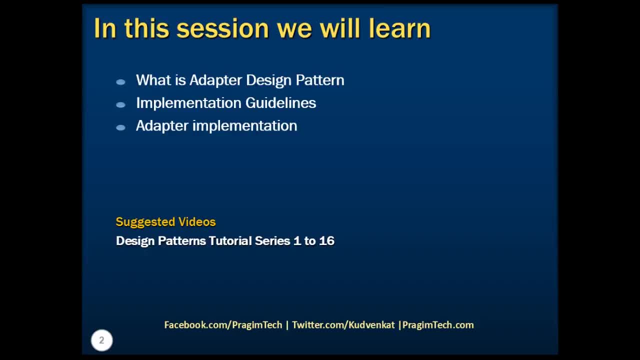 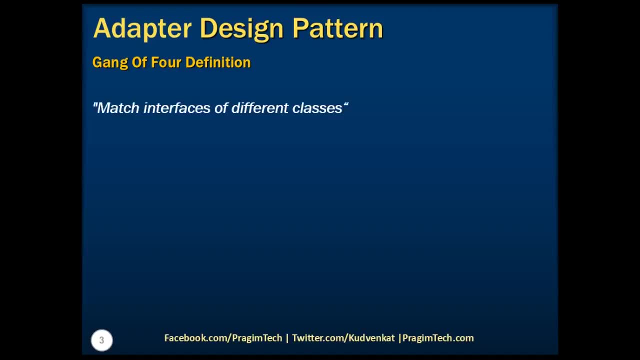 to the previous parts of the tutorial before proceeding. As per the Ganga 4 definition, adapter match interface of different classes, which means an adapter allows two incompatible interfaces to work together. In software engineering, the adapter pattern is a software design pattern that allows the interface of an existing class to be used from another interface. 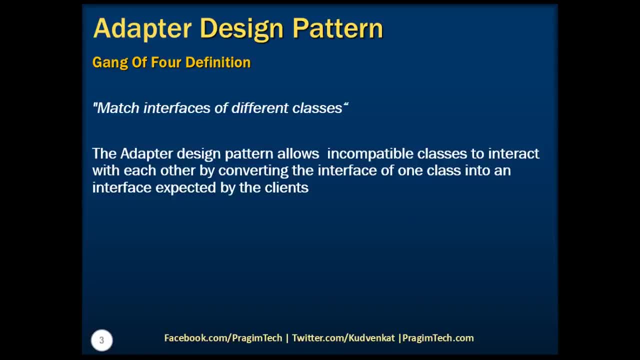 It is often used to make an existing classes work with others without modifying their source code. Leveraging on adapter pattern improves reusability of older functionality. Having said that, adapter pattern works as a bridge between two incompatible interfaces, which means this type of design pattern comes under structural pattern, as this pattern combines the capability of 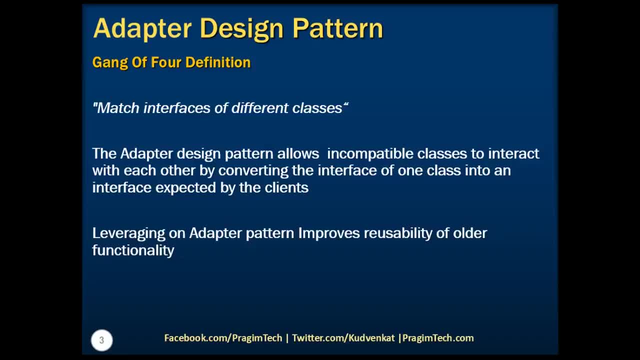 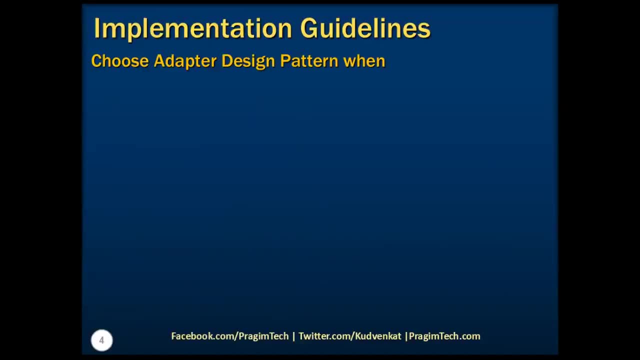 two independent interfaces. Now the question comes: when do we need to choose adapter design pattern? We can say that adapter design pattern is a design pattern that is adapted to a specific class. We need to choose adapter design pattern when a class needs to be reused that doesn't have an interface that a client expects. Also, when we need to work through 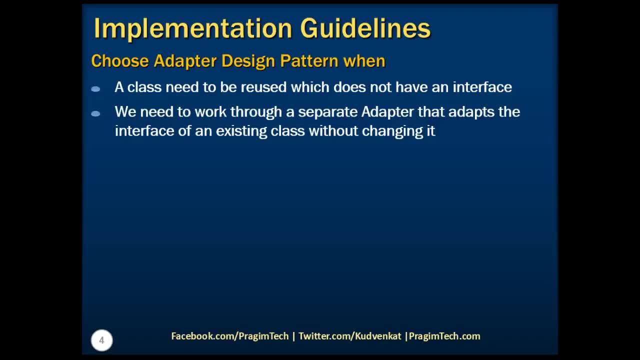 a separate adapter that adapts the interface of an existing class without changing it. Also, we need to choose this pattern when client don't know whether they work with a target class directly or, through another adapter, with a class that doesn't have the target interface. 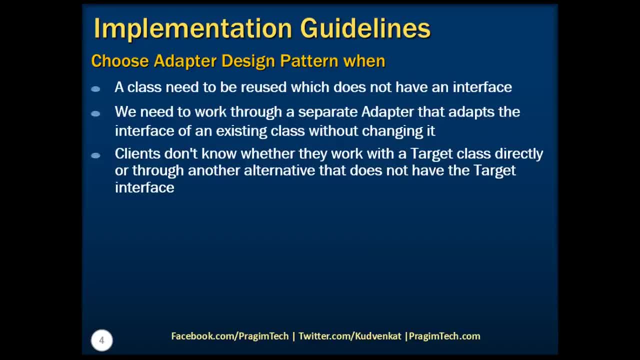 I am sure this is confusing at this moment, but don't worry, we will take a look at this with an example. Now, when we talk about example, the perfect example of a adapter design pattern is the AC adapter. The AC adapter knows how to deal with both sides, isn't it? It acts as a middleman. 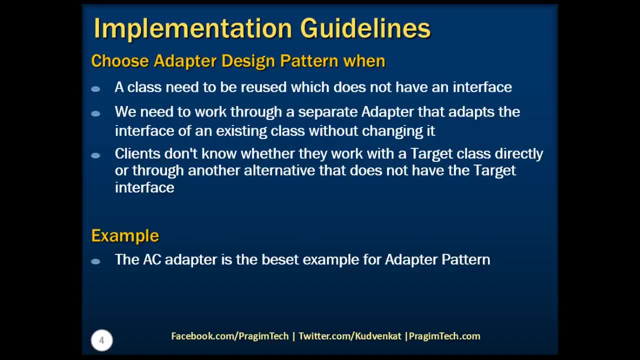 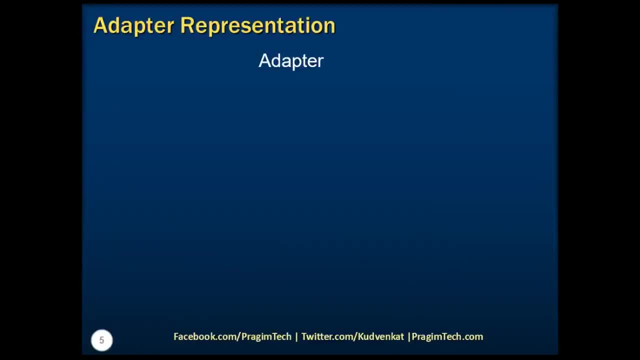 between two sockets. That is a perfect example of adapter design pattern. Let's now take a look at the representation diagram of adapter design pattern. The client class over here is used to communicate with adapter class that implements the iTarget interface. In other words, this is: 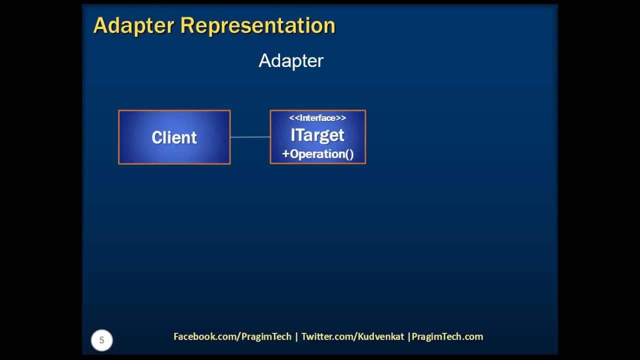 the class used for creating the instance of adapter class. Now, the iTarget here represent an interface created to make client achieve its purpose, Whereas the adapter class implements the iTarget interface and inherits the Adaptee class as well. Hence we can see that this works as mediator. 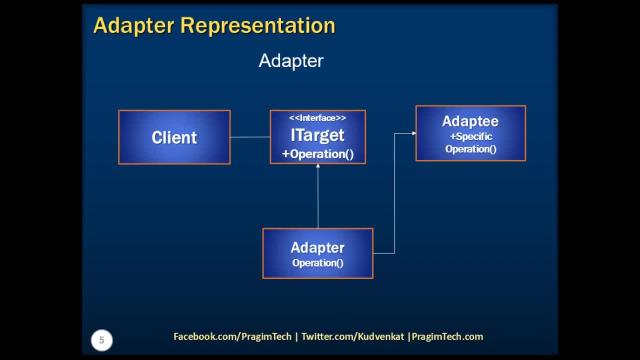 between iTarget interface and Adaptee class. Finally, the Adaptee class contains the main functionality that a client is expecting. Let's now switch to version 1.. Let's go back to visual studio and understand the adapter design pattern with a very simple example. 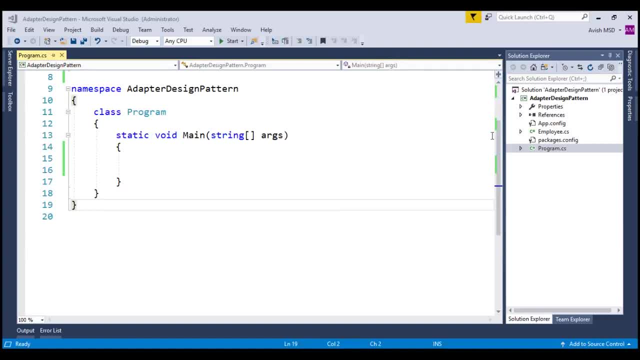 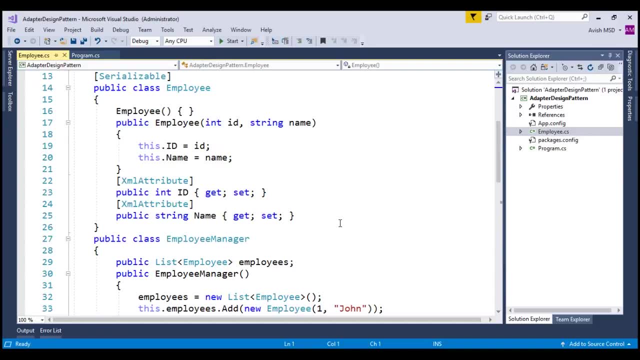 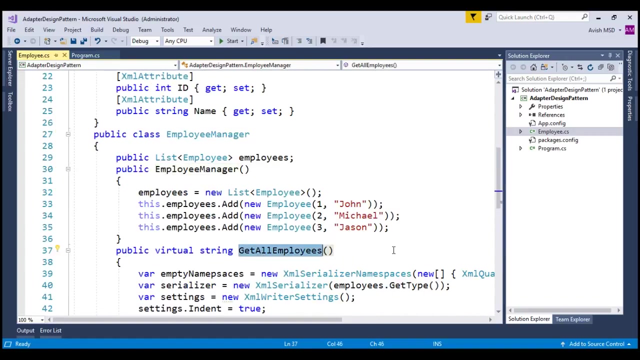 To save some time, I have already created a console application which has employee and employee manager classes. Employee class has properties of employee id and employee name. This is basically a very simple employee class. Now the employee manager has a method called getAllEmployees that returns all the employees as XML string. 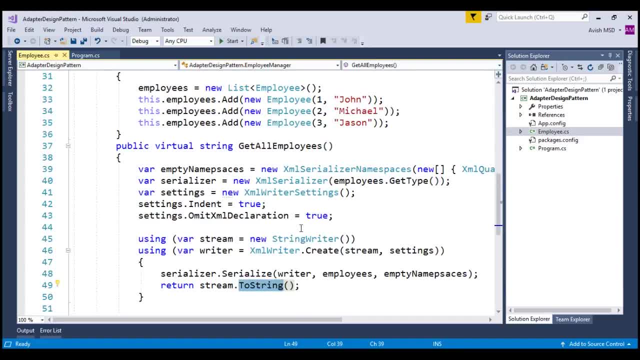 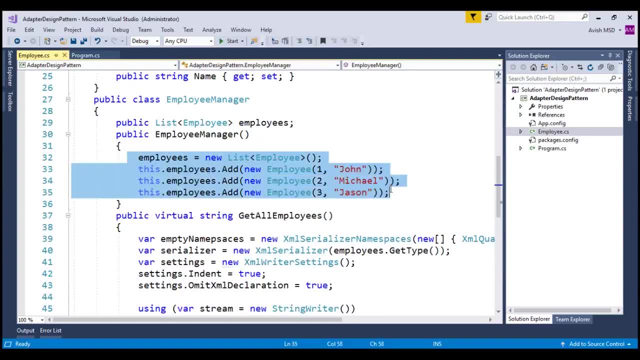 Before returning the employees. we assume that the employees are already present in the system. To simulate that I have created few employees in the constructor of this class. Now it looks all perfect till this moment. What if I need details related to employees in JSON format? 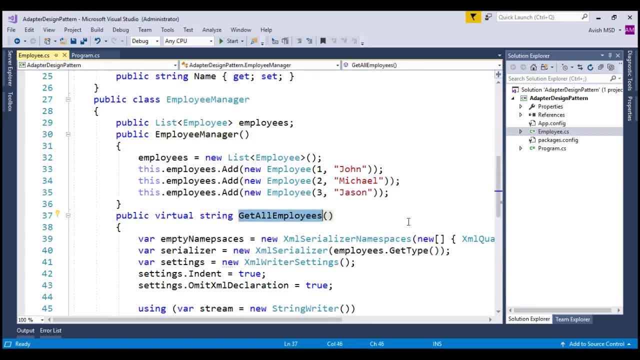 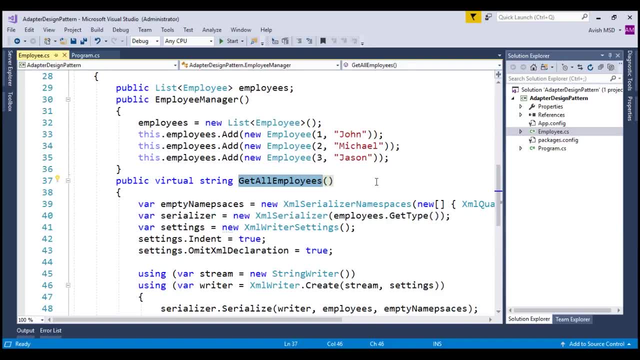 instead of XML format. To achieve that, I cannot use this method directly, but somehow I need to leverage on this method to get the employee details in JSON format. That means we need to create some more interfaces and classes that a client can leverage on to reuse the existing. 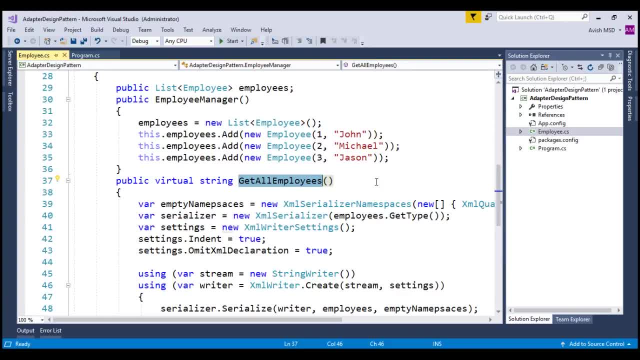 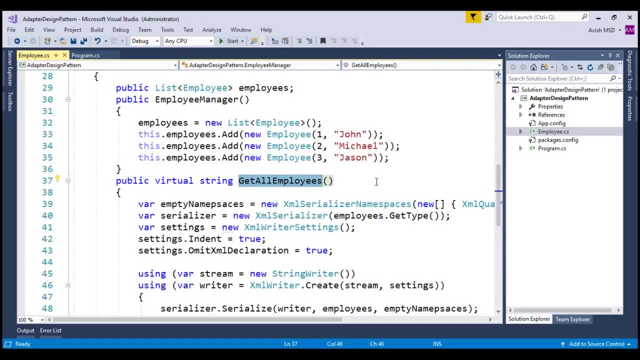 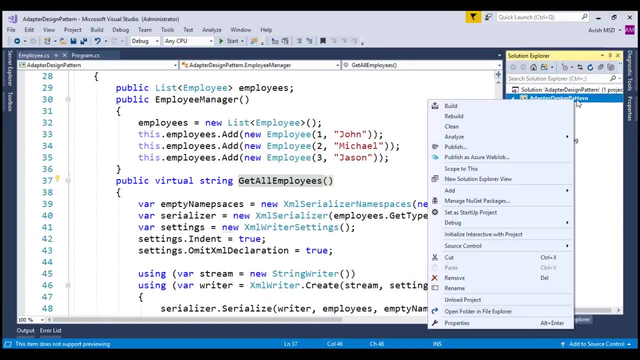 adaptive class. I repeat: This need to become an adaptive class and we need to create adapter to combine two incompatible request and responses. To achieve that, let's create an interface and name it as IEmployee. Right click on this project, add new item, choose an interface and name this as IEmployee. 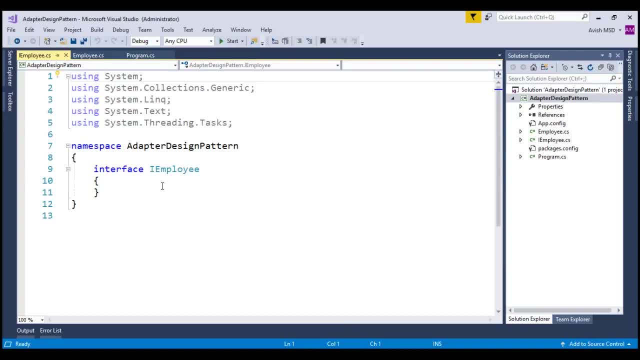 This IEmploy interface returns the getAllEmployee details in the form of JSON, which means IEmploy interface serves as target for the client to interact. So let's create a method which returns a string which is getAllEmployees. Let's also make this interface as public. 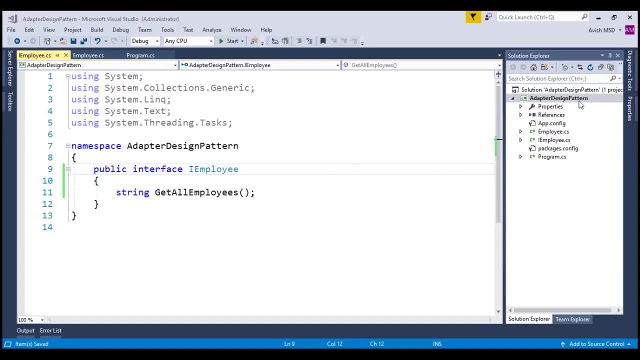 Let's now create a new folder. right-click add new folder and name this folder as target. Let's move this IEmployee into the target folder. It's not mandatory to create folders and move these classes or interfaces under these folders. I'm following this folder structure presentation to make this example simple to understand. 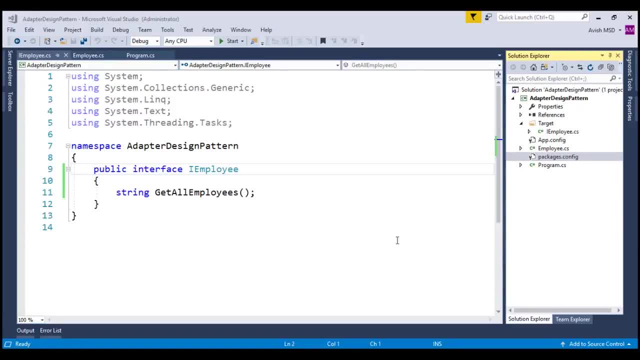 based on my experience. Let's move this file into our representation diagram. Let's right-click and add new folder and name this folder as adaptee. As mentioned earlier, the employee and employee manager are adaptee over here. Let's move this class file under adaptee folder. 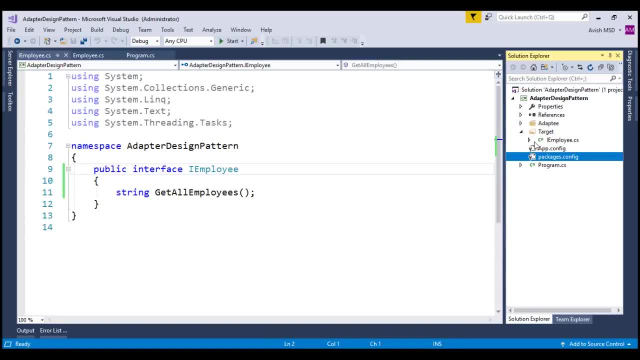 Let's click on OK. So we now have adaptee and target related classes. We need to create adapter classes related classes. let's right click on this project, add new folder and name this folder as adapter. let's right click on this adapter folder, add new item and. 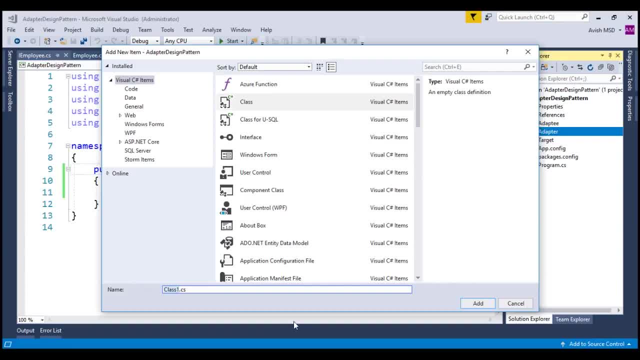 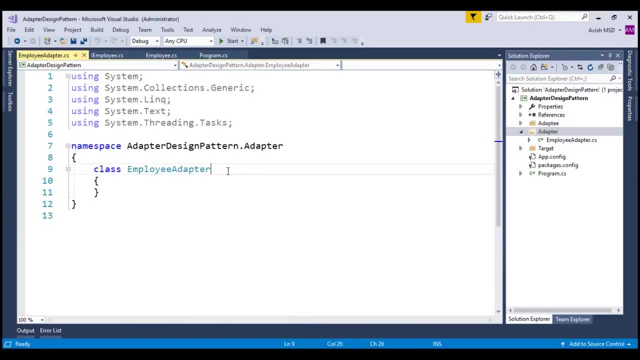 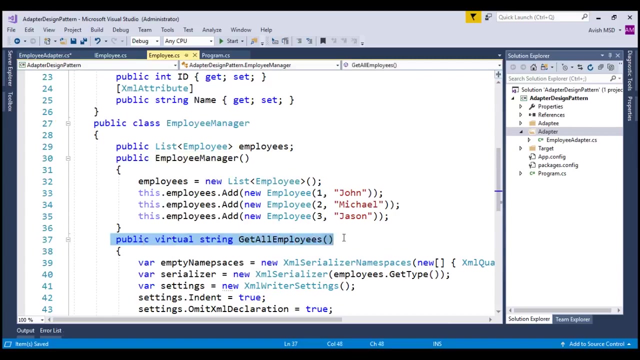 choose a class and name this class as employee adapter. this employee adapter class implements the employee manager as well as inherits the I employee. let's make this class as public and let's overwrite the method of the employee manager. if you notice that we have created this method as virtual method, so 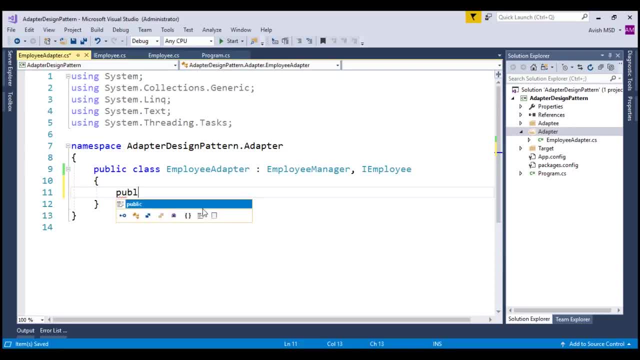 let's overwrite this virtual method. public overwrite- get all employees. so let's say string: get all employees. look at that, it has pre-populated the details. instead of returning the base, dot: get employees. we need to change the XML to JSON and return it back. let's see how we can do. 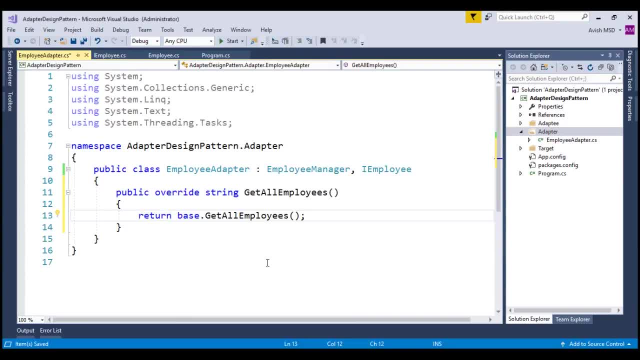 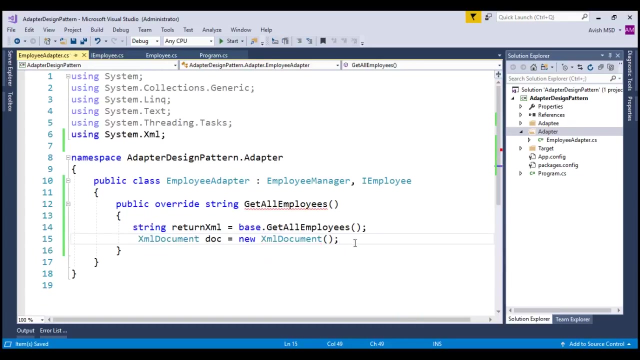 that let's create a variable called string return XML equal to base dot get employees. now that we have this XML, we need to convert this XML to JSON. let's create XML document, name it as doc, equal to new XML document. let's resolve these issues by using system dot XML and let's load this written XML into this document. 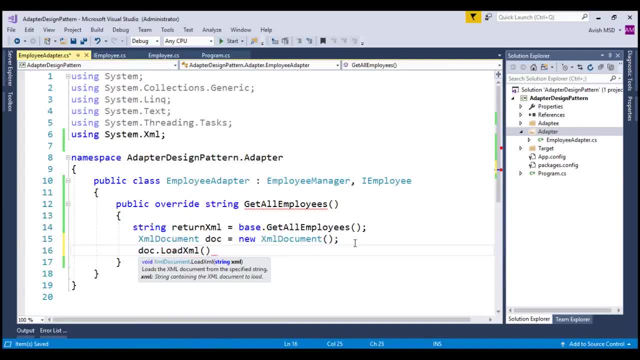 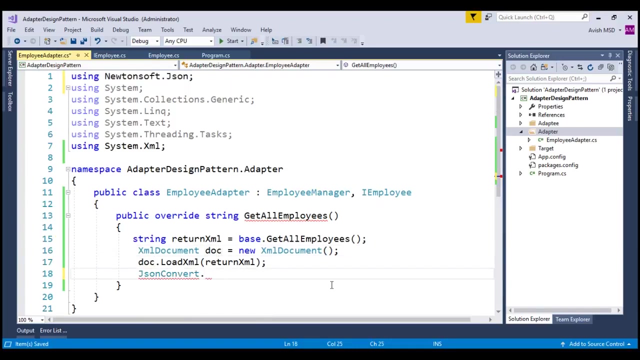 document dot, load XML and say written XML. now we can use the Newton's of Jason over here and convert this XML to JSON string. let's say: Jason, convert dot. let's resolve this issue by using Newton's of dot Jason and say: serialize object by passing this document: comma Jason. 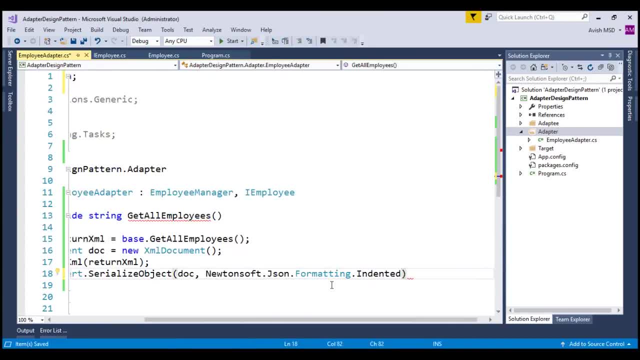 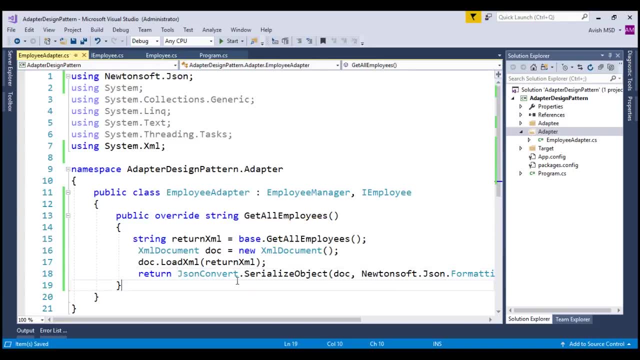 serialization formatting: dot indented. we need to return this Jason string as per the requirement, so let's return it back. let's format this method. now that we have created adaptive, adapter and target related classes and interfaces, let's invoke the adapter from the client. let's switch to the main program. to save some time, I have already kept the code. 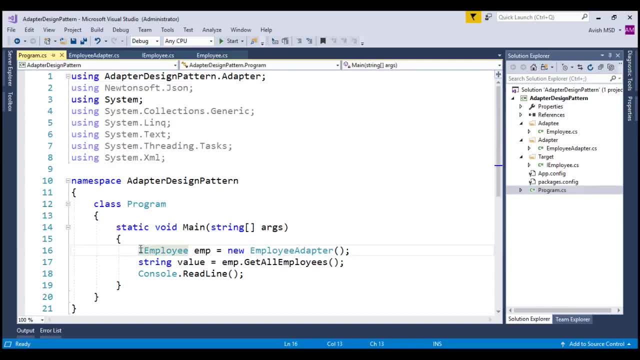 ready in the client program. notice that using the target interface and use vamos, which is I employee, or here we are creating a new employee adapter class and invoking the get employee details. now let's run this application and step to the code to see if we are able to retrieve the JSON details of the 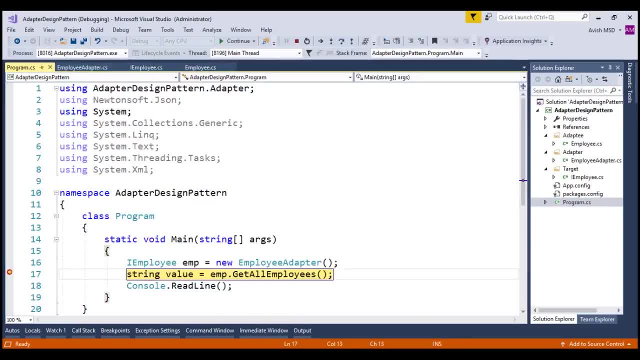 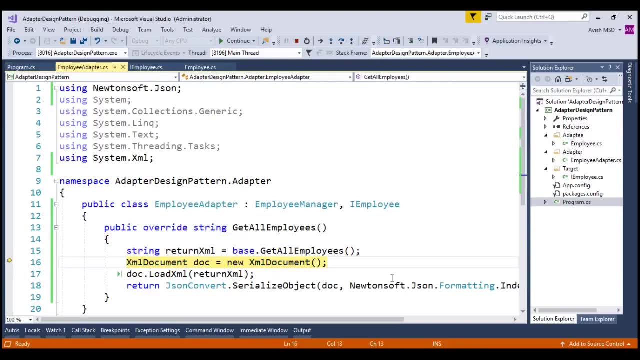 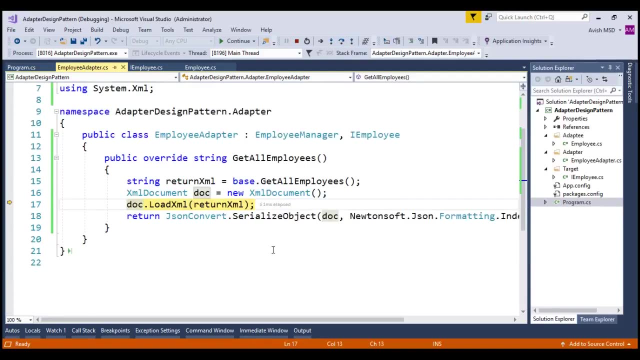 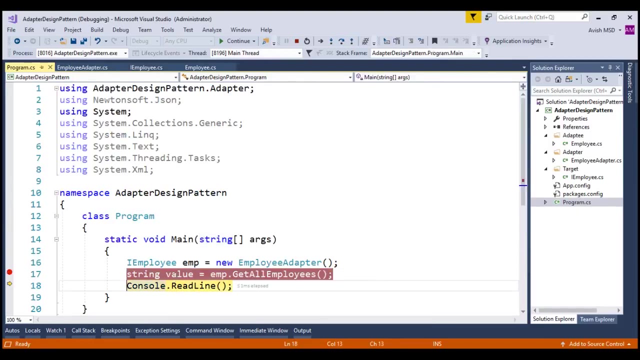 employee. let's just put a breakpoint over here. let's run this application, let's step into the get employees notice that we are calling the base dot get, returning the XML file, and the XML document which we have written over here is loading the XML and using the JSON convert, we are converting this XML into.